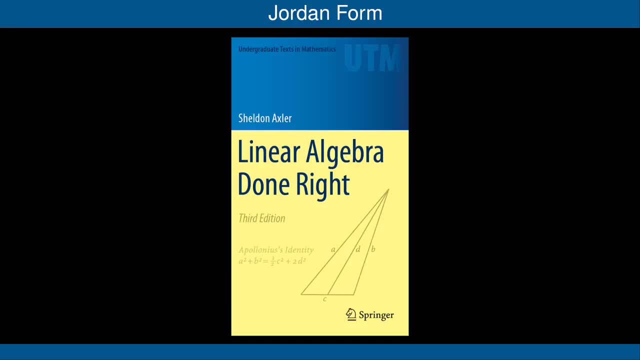 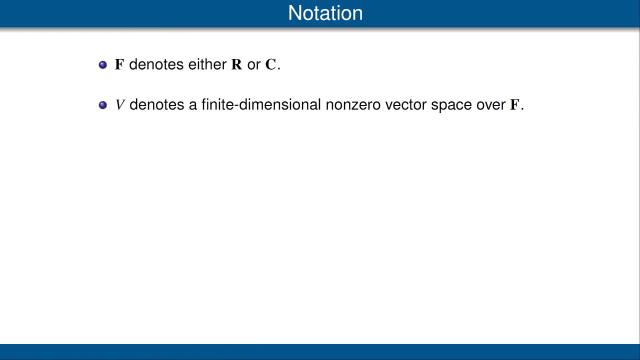 Hello, I'm Sheldon Axler, the author of Linear Algebra Done Right. This video discusses the section of the book titled Jordan Form. Let's quickly review our standard notation. F denotes either the scalar field R of real numbers or the scalar field C of complex numbers. 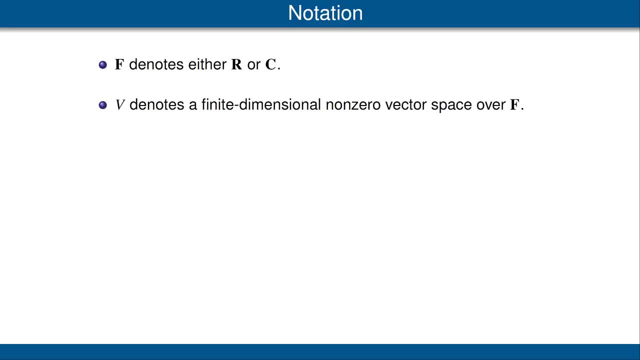 V always denotes a finite-dimensional, nonzero vector space over F. Suppose V is a complex vector space and T is an operator on V. Earlier in these videos we proved that there's a basis of V with respect to which T has an upper triangular matrix. 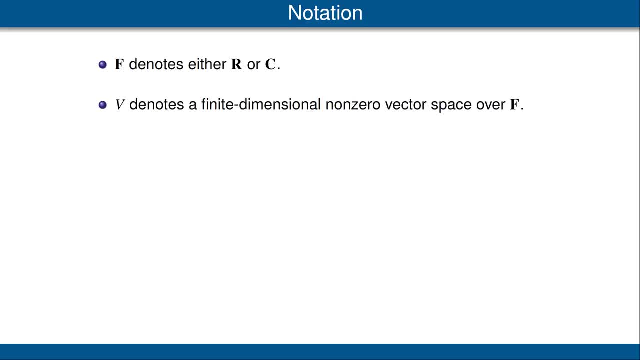 Later, we proved something called the decomposition theorem. that gave us not only a basis with respect to which we have an upper triangular matrix, but we got considerably more zeros than we might have expected. Now, in this video, we're going to do even better. 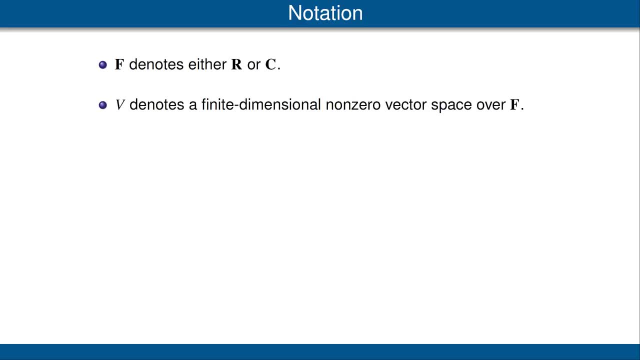 We're going to show that there's a basis of V with respect to which the matrix of T is zero everywhere, except possibly along the diagonal and the line directly above the diagonal. Let's start with some examples so we can get a feeling for what's going on. 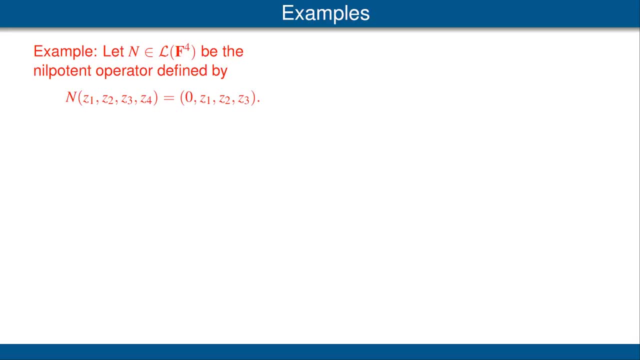 Let N be the operator on F4, defined by the equation that you see here. You should pause the video for a moment to verify that N is a nilpotent operator. Now let V be the vector. Then you should verify that N cubed applied to V and squared applied to V. N of V, V. 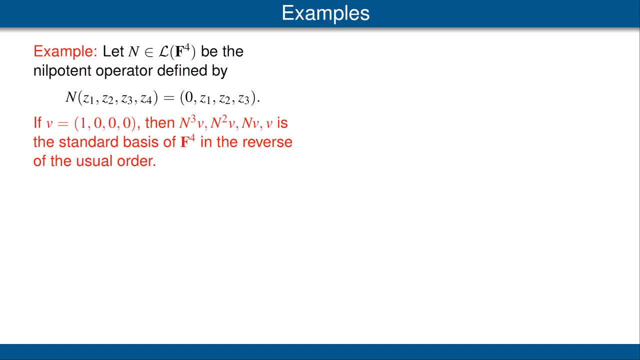 is just the standard basis of F4, but in reverse of the usual order, And you should also verify that- the matrix of N with respect to this basis is the matrix shown here. Zeros everywhere, except ones directly above the diagonal, Because N is nilpotent. we know that zero is the only eigenvalue of N. 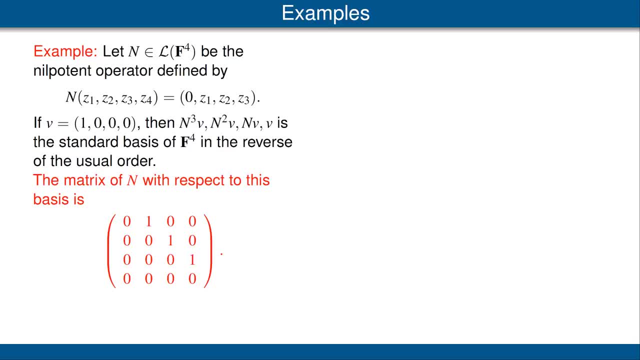 Thus, if we choose a basis with respect to which N has an upper triangular matrix, we know that the entries along the diagonal will be all zeros, But we've done a little better here, with ones on the line directly above the diagonal and zeros everywhere else. 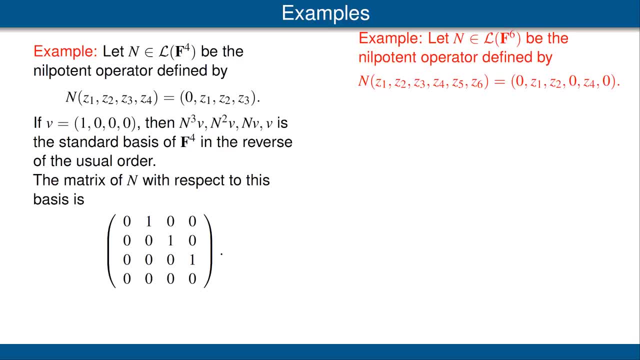 Now let's look at another example. Let N be the operator on F6 defined by the equation you see here. Please pause the video and verify that N is a nilpotent operator. You might think from the previous example that we can find a basis of F6,. 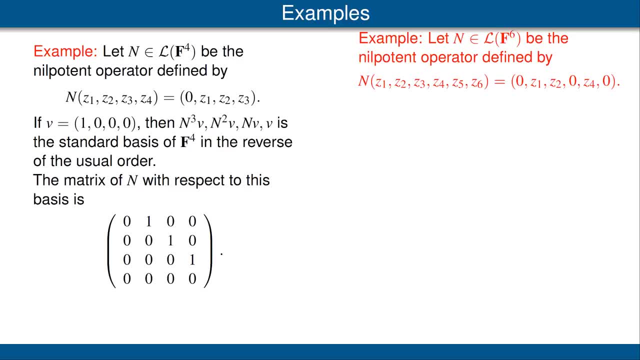 such that the matrix of this operator N, with respect to that basis, contains only ones on the line directly above the diagonal. However, that's not possible with this operator. Here's what we can do, however. Let V1,, V2, and V3 be the vectors shown here. 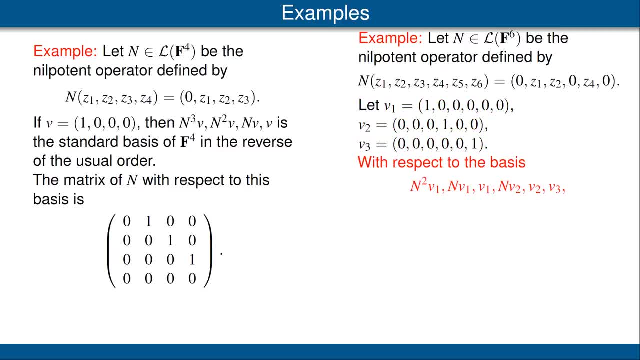 You should pause the video to verify that this list, namely N squared of V1, N of V1, V1, N of V2, V2, V3, that that list is a basis of F6.. Now you should also verify that the matrix of N. 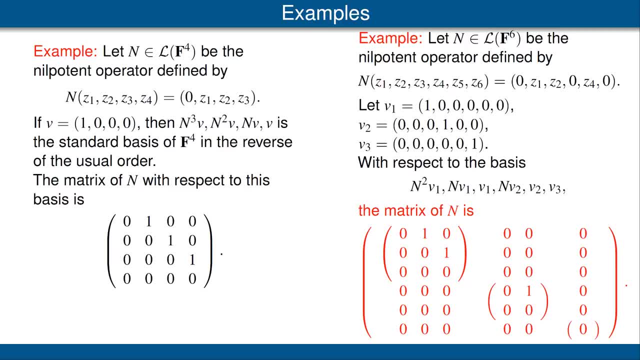 with respect to that basis is the matrix shown here. This is a 6x6 matrix, as expected, but I've inserted some extra parentheses to show that we can think of this as a block-diagonal matrix And each of the blocks has the form of the previous example. 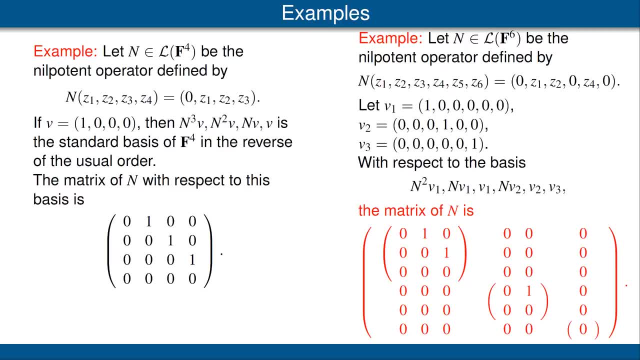 The first block is a 3x3 matrix with ones above the diagonal and zero everywhere else. The next matrix is a 2x2 matrix with ones in the line above the diagonal, which is just one entry, And the last one is a 1x1 matrix containing zero. 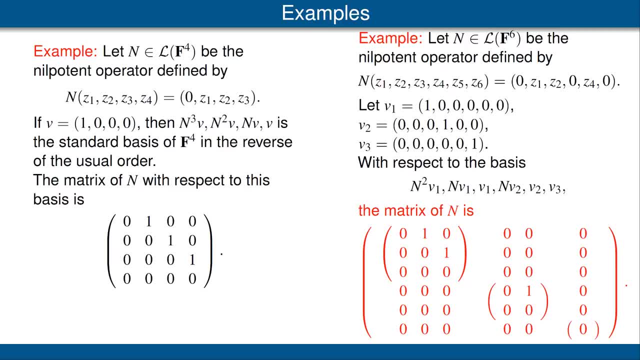 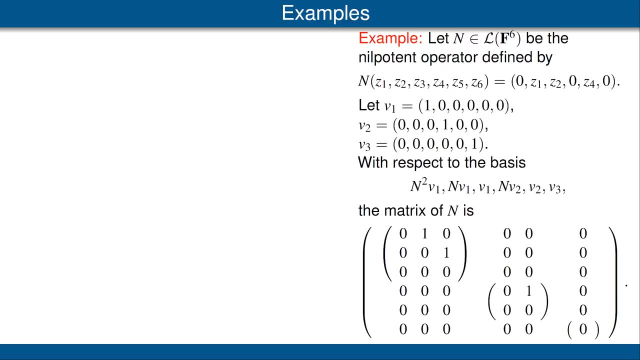 There are no entries here, above the diagonal. Our next result states that we can always do something like this for any nilpotent operator. Let's erase the first example, but leave the second example on the slide so that it can illustrate the theorem. 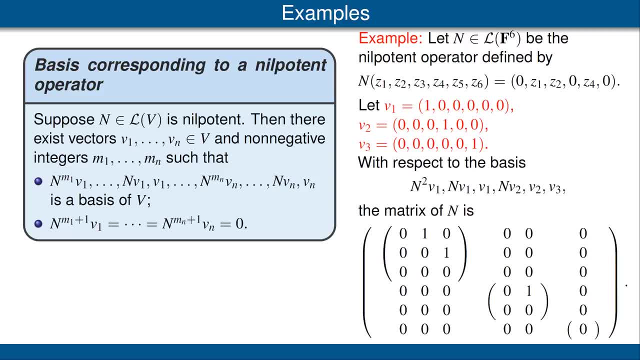 Here's the result. This result is the heart of the Jordan form. Here's what it says. Suppose N is a nilpotent operator on V, Then there exist vectors v1 up through vN, and think in terms of the example v1 up through v3,. 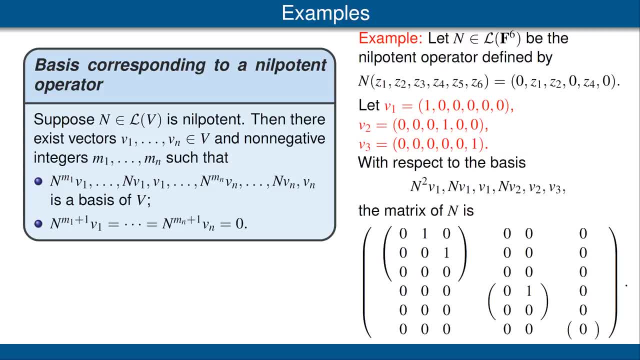 which are now highlighted in red on the right, And there exist non-negative integers, m1 up through m sub N, And for the example now highlighted in red, we see that those numbers are 2,, 1, and 0.. And the conclusion, first bullet point on the left. 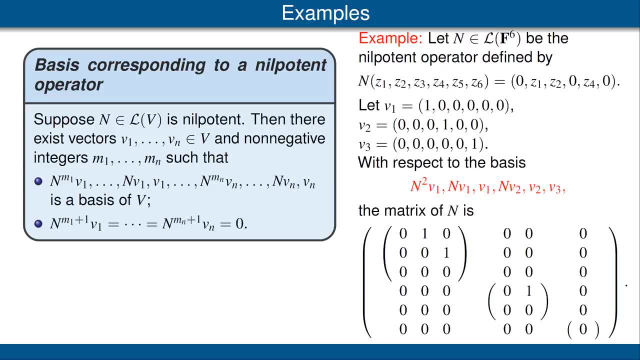 is that those vectors form a basis of V, just as we see a basis of V in red on the right-hand example. And then the second bullet point says: if we want one higher integer and apply it to all those vectors, we would get zero. 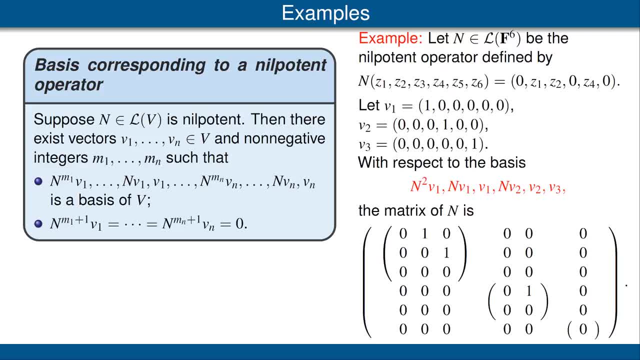 And again you can see that that's the case in the example. If you pause the video, read this theorem several times, compare it to the example and make sure you understand what it's saying. Now that you're back from understanding what this result says, 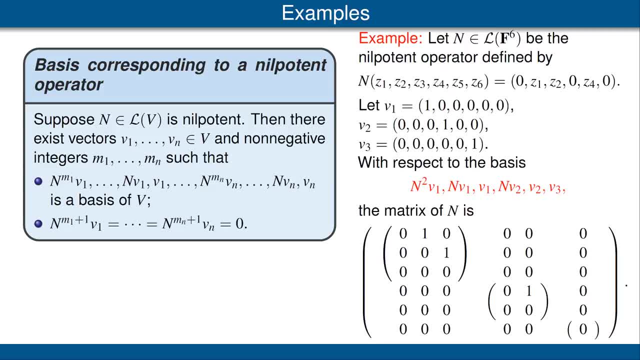 you may want to look at the proof, which we're not going to do in this video. To see the proof, look in the book. I will tell you that the proof is by induction on the dimension of V. Before we leave this slide, 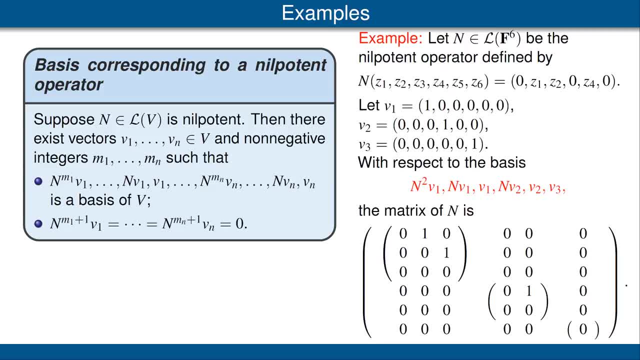 it's important that you understand what the matrix of N looks like with respect to the basis given in the first bullet point. The first basis vector is N to the power m1 applied to V1.. To see the first column of the matrix of N: 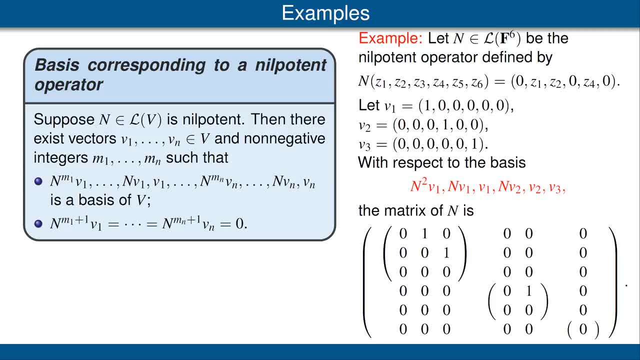 we apply N to that first basis vector, We get N to the power m1 plus 1 applied to V1, which, by the second bullet point, is zero. Thus the first column of the matrix of N with respect to this basis, is only of zeros. 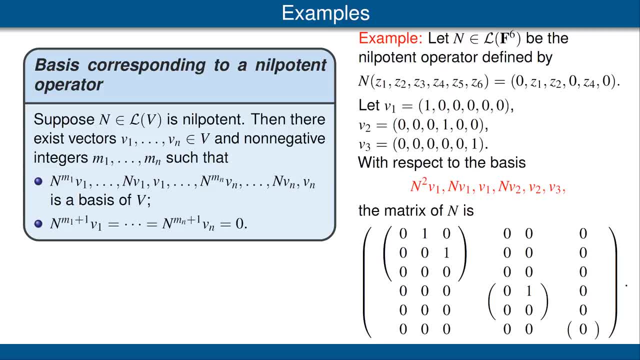 Let's assume that m1 is positive, just for the purposes of this example. Then if we apply N to the second basis vector in our list, in the first bullet point, we get the first basis vector. That means the second column consists of 1. 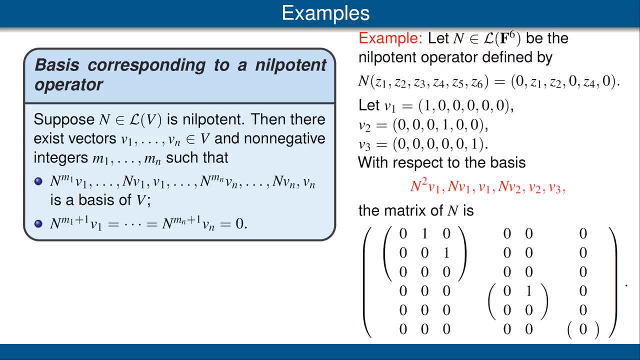 followed by all zeros And so on. In other words, the matrix of N with respect to the basis shown in the first bullet point looks very much like the matrix shown to the right in the example. Specifically, we get a block-diagonal matrix. 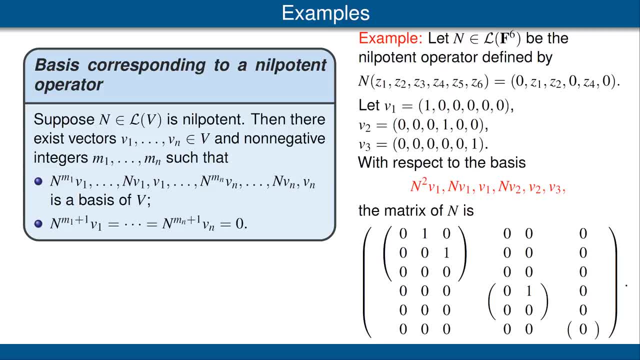 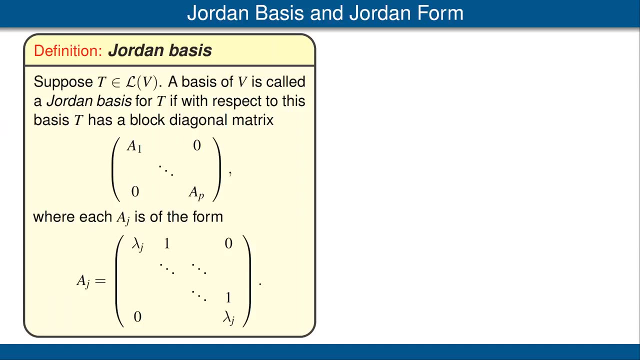 where each of the matrices on the block-diagonal consists of zeros, except for the line directly above the diagonal, which consists just of ones. Please pause the video and make sure that this is clear to you. We have been discussing nilpotent operators. 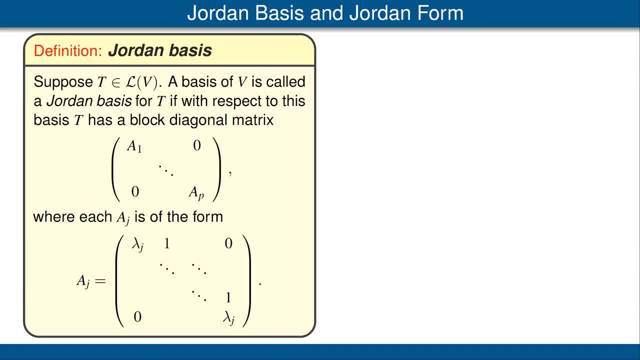 It's time now to discuss more general operators. Using as motivation what we just learned about nilpotent operators, we make the following definition: Suppose T is an operator on V, A basis of V is called a Jordan basis for T. if, with respect to this basis, 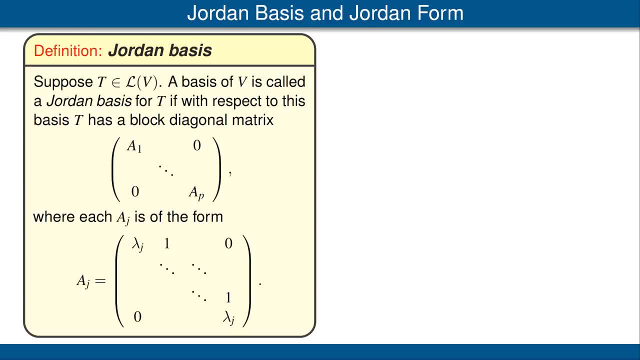 T has a block-diagonal matrix where each of the entries on the block-diagonal consists of all zeros, except for some constant along the diagonal and ones above the diagonal. The constant along the diagonal can change depending upon which block you're in, but within each block. 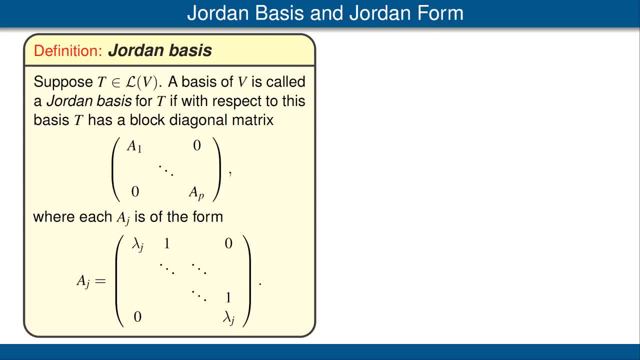 just constant lambda sub j along the j-th diagonal constant, one above the diagonal zeros everywhere else. The result that we discussed on the last slide implies that each nilpotent operator has a Jordan basis where all the lambda j's are equal to zero. 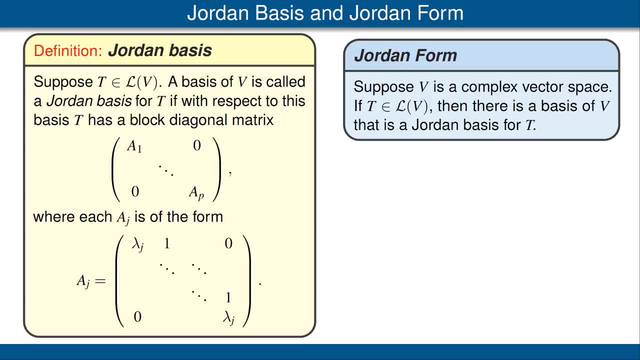 Now we come to the Jordan form theorem as the culmination of the results we've discussed previously in this video. Suppose V is a complex vector space. If T is an operator on V, then there's a basis of V that is a Jordan basis for T. 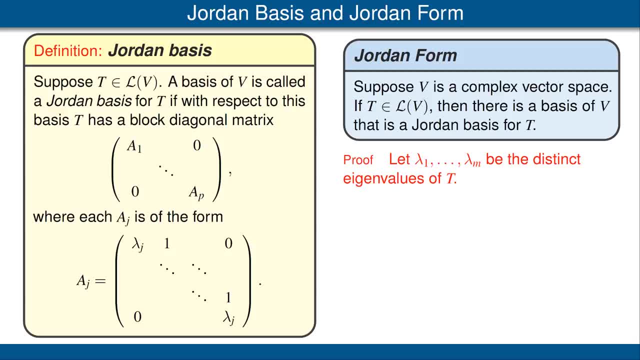 Let's look at the proof of this result. We start by letting lambda 1 up to lambda m be the distinct eigenvalues of T, We have the generalized eigenspace decomposition writing V as the direct sum of the generalized eigenspaces corresponding to those distinct eigenvalues. 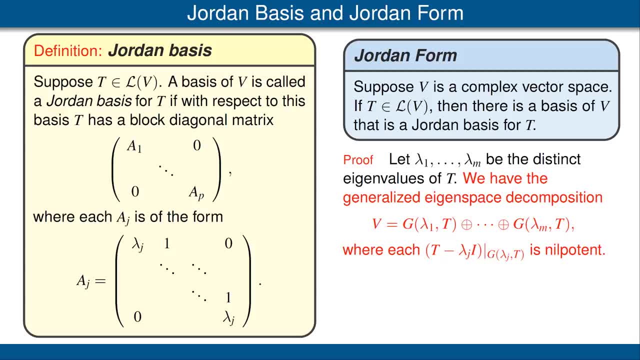 This is where we use the hypothesis that V is a complex vector space, because this decomposition is not necessarily true if V is a real vector space. Our decomposition theorem said that T minus lambda j times the identity operator when restricted to the generalized eigenspace. 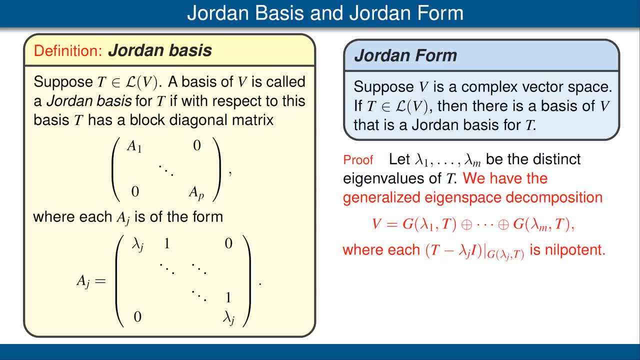 corresponding to the eigenvalue lambda j is a nilpotent operator. Thus, by the results we have been discussing, some basis of each generalized eigenspace is a Jordan basis for T minus lambda j, i restricted to the corresponding generalized eigenspace.